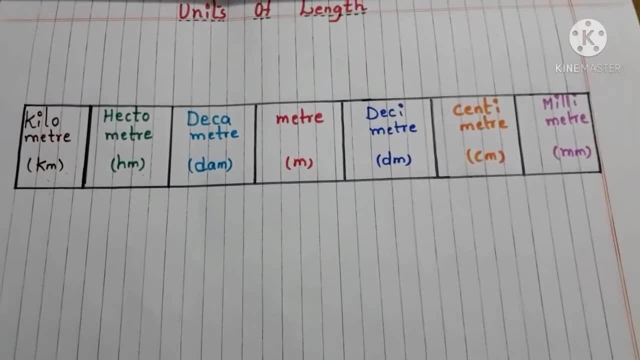 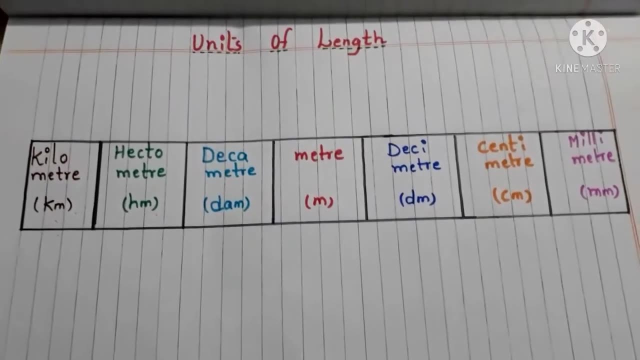 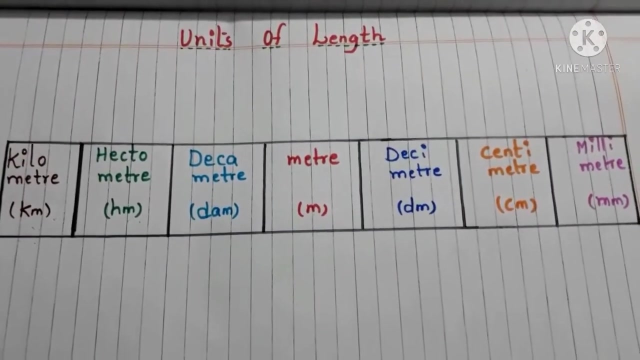 Now let us see how to convert the length from one unit to another unit. Here we have to remember two important points: Whenever we want to convert the highest unit to lowest unit, we have to multiply. Or else, whenever we want to convert the lowest unit to highest unit, we have to divide. 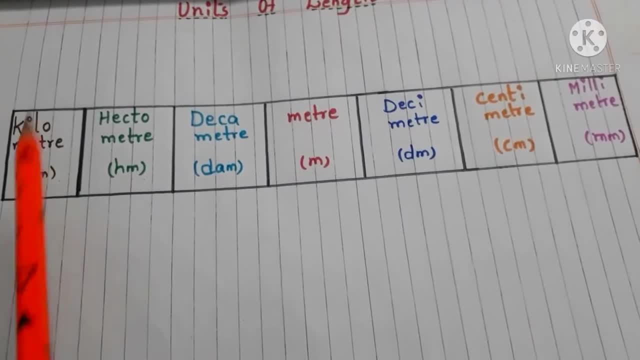 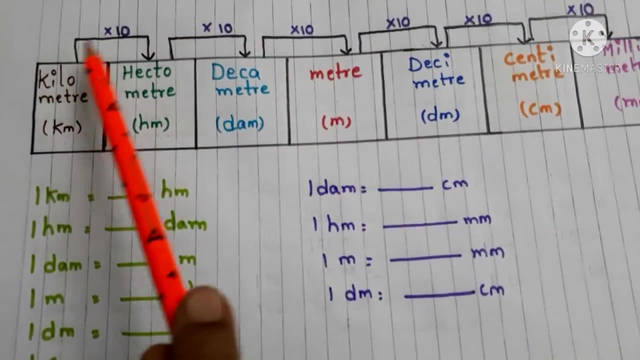 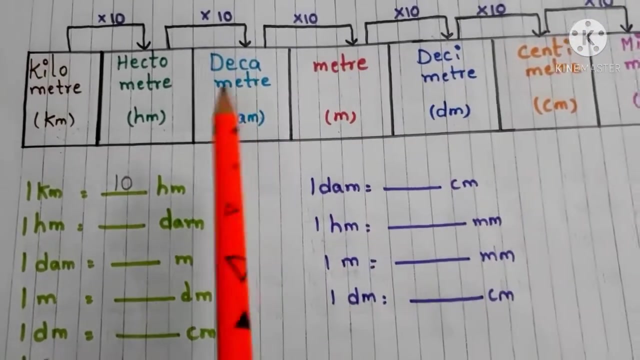 First, let us see how to convert highest units to lowest units. If we want to convert kilometers into hectometers, we have to multiply with 10.. Means that 1 kilometer is equal to 10 hectometers. If we want to convert hectometers to decameters, again we have to multiply with 10.. 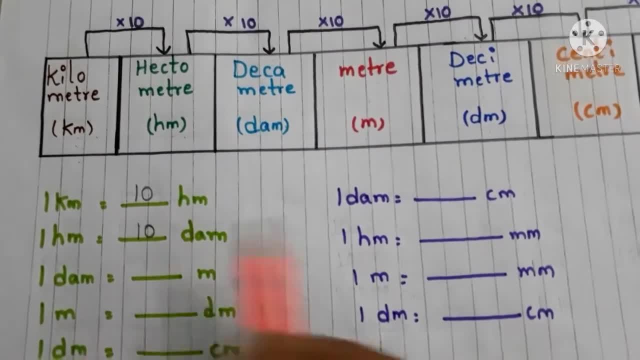 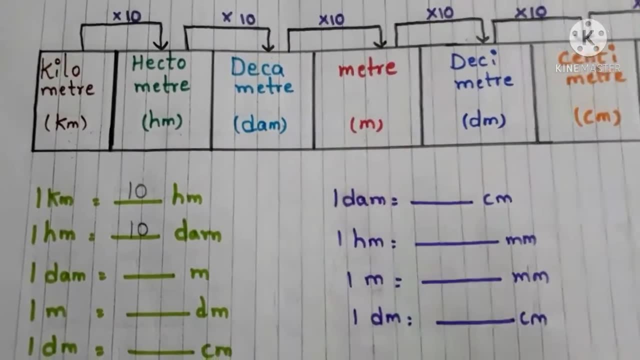 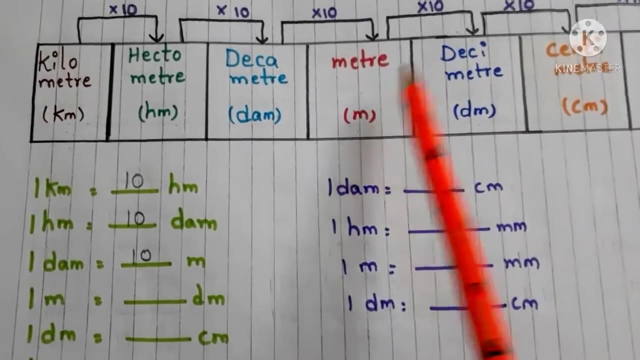 Means that 1 hectometer is equal to 10 decameters, And if we want to convert decameters into meters, we have to multiply with 10.. Means that 1 hectometer is equal to 10 decameters, And if we want to convert meter to decameters, we have to multiply with 10.. 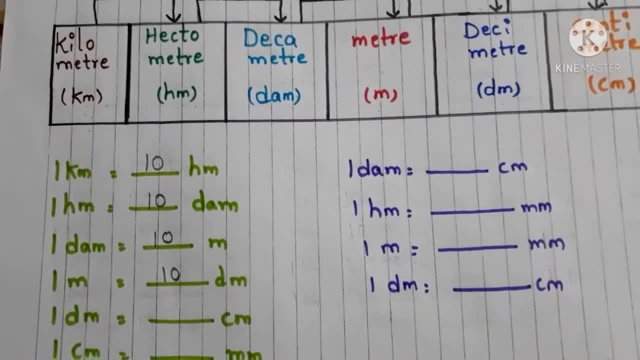 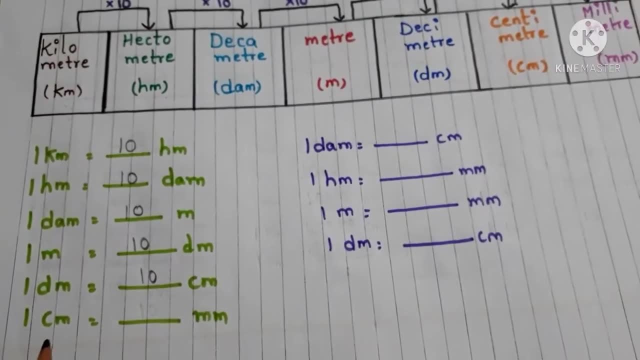 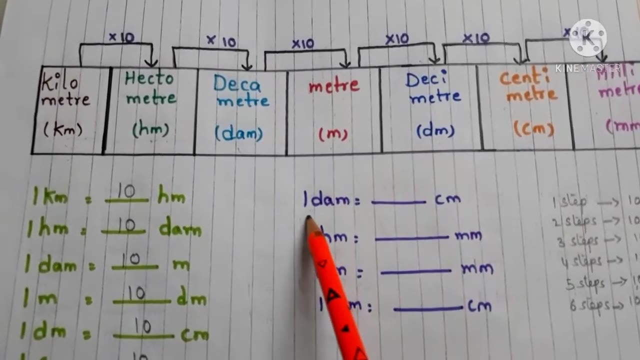 Means that 1 meter is equal to 10 decameters. Like that, 1 decameter is equal to 10 centimeters. 1 centimeter is equal to 10 millimeters. Okay, Now let us see 1 decameter is equal to how many centimeters. 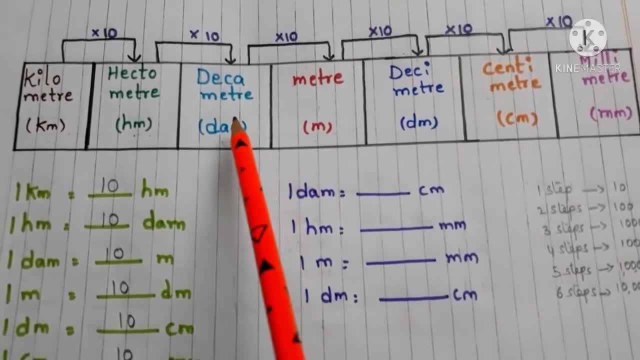 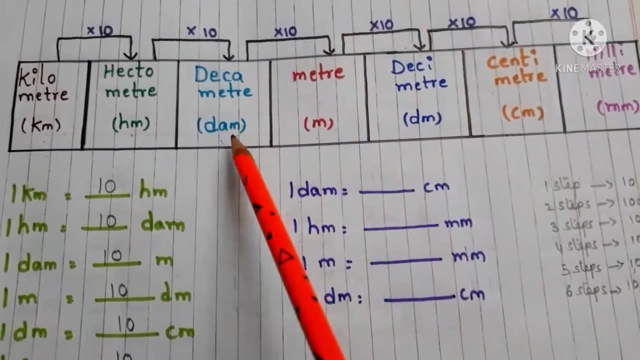 Where is decameter in the table? Here it is. Where is centimeter in the table? Here it is How many steps we have to move from decameter to centimeter. Let us see 1,, 2,, 3.. 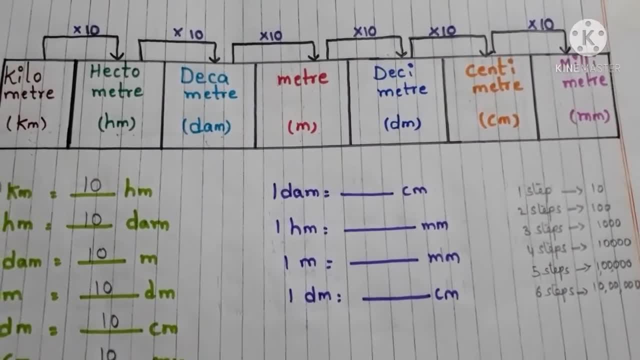 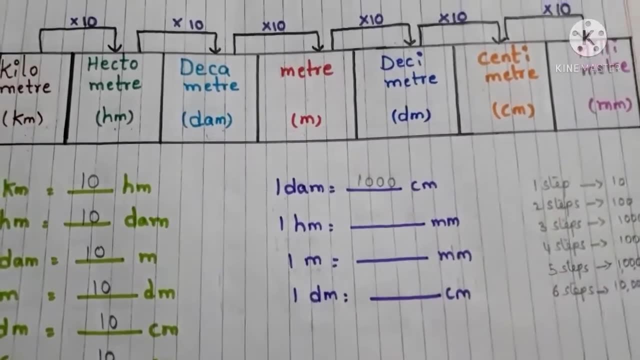 3 steps. we have to move, So we have to multiply with 1000.. Means that 1 decameter is equal to 1000 centimeters. Okay, Okay, 1 hectometer is equal to how many millimeters? 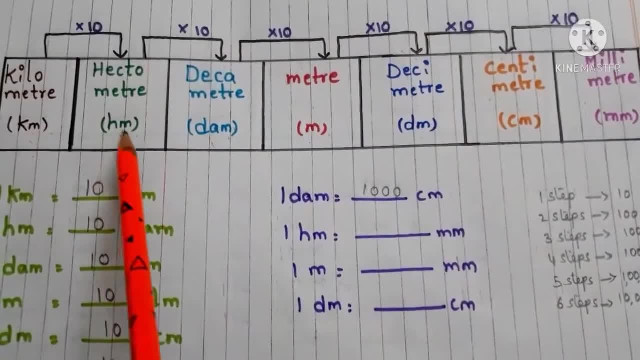 1 hectometer is equal to how many millimeters? Let us check. Where is hectometer in the table? Here it is. Where is millimeter in the table? Here it is How many steps we have to move. Let us see. 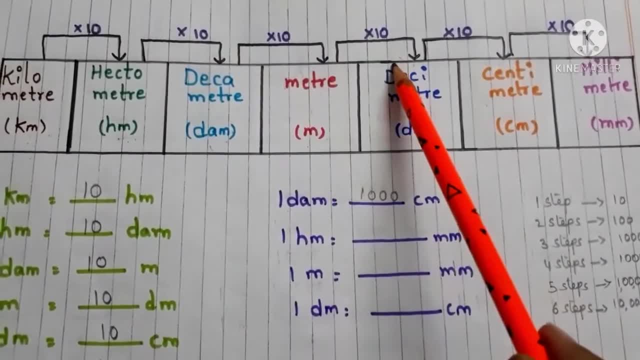 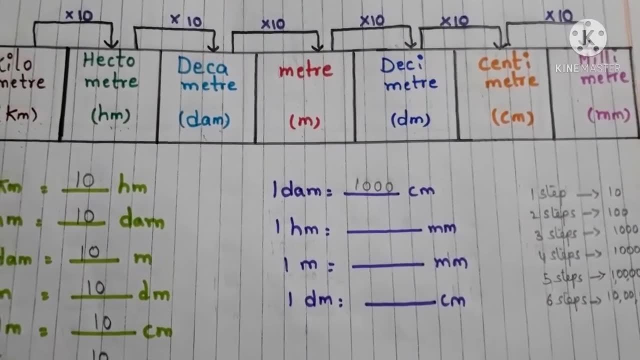 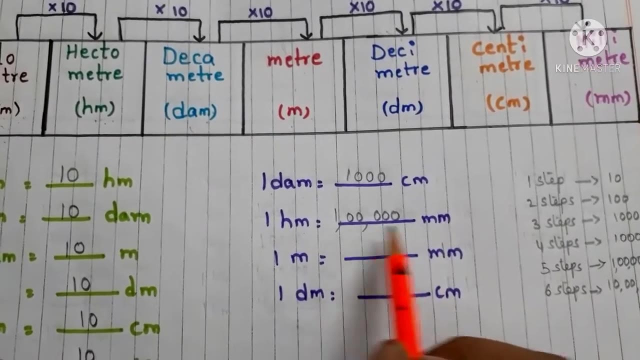 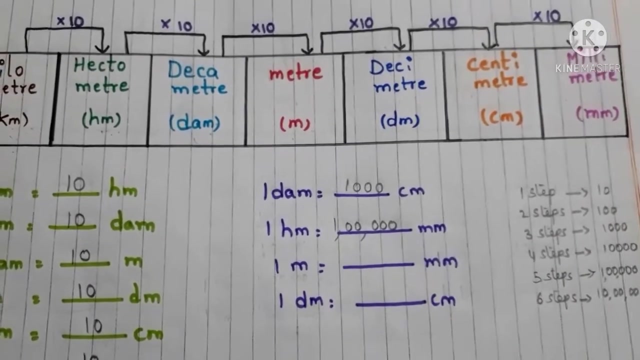 1, 2, 3, 4, 5.. 5 steps we have to move. So we have to multiply with 1. lakh Means that 1 hectometer is equal to equal to 1 lakh millimeters. Okay, 1 meter is equal to how many millimeters? Let us see in the 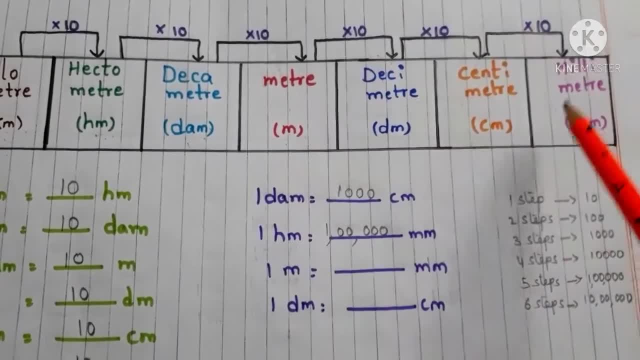 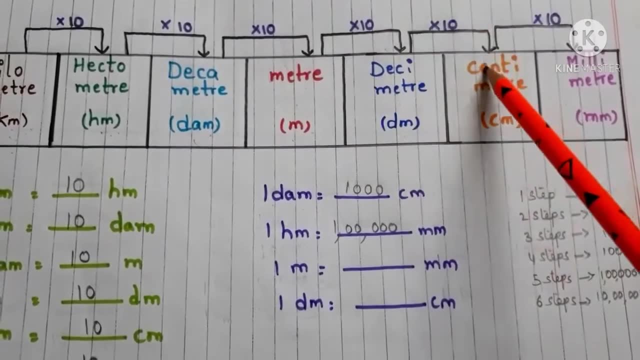 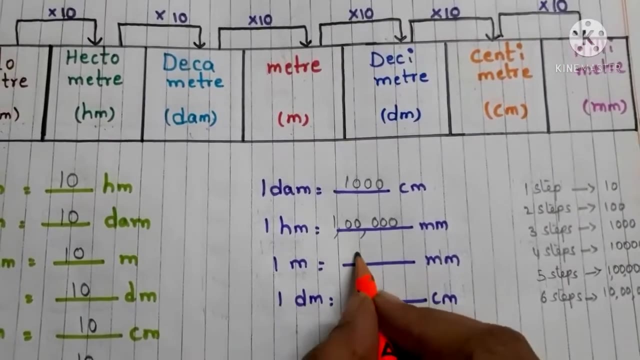 table. Where is meter? Here it is. Where is millimeter? Here it is How many steps we have to move. See 1, 2, 3.. Three steps Means we have to multiply with 1000.. Means that 1 meter is equal. 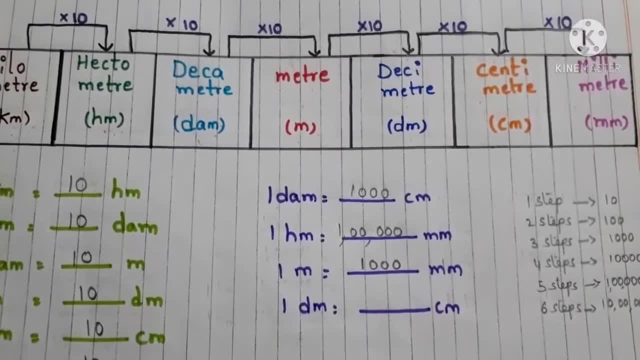 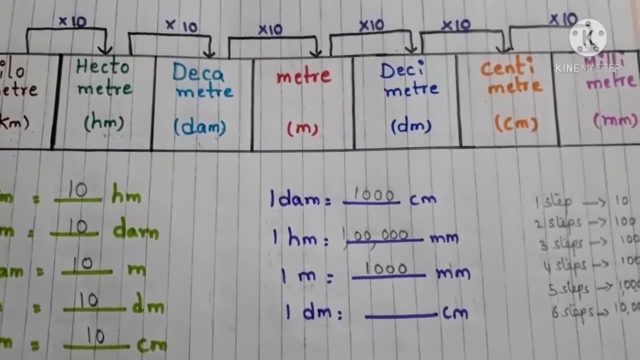 to 1000 millimeters. Okay, 1 decimeter is equal to how many centimeters? Let us see in the table. Where is decimeter in the table? Here it is. Where is centimeters? Here it is. So we have to move. 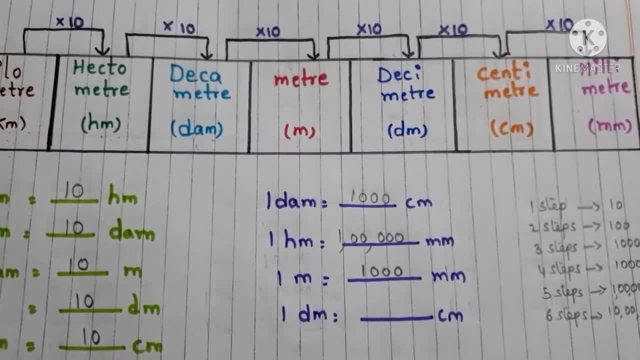 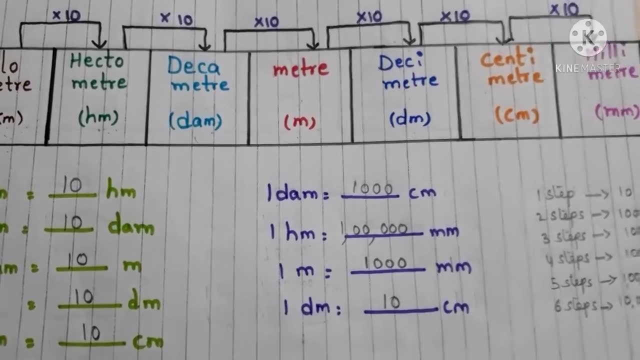 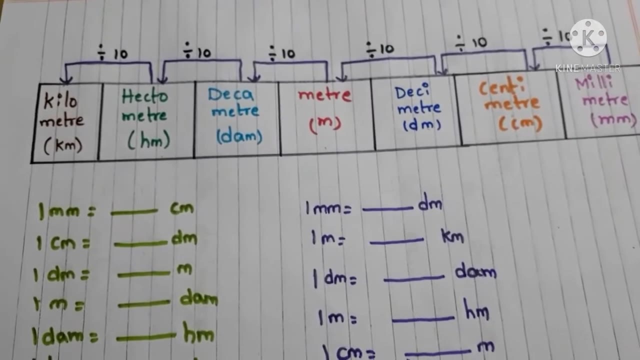 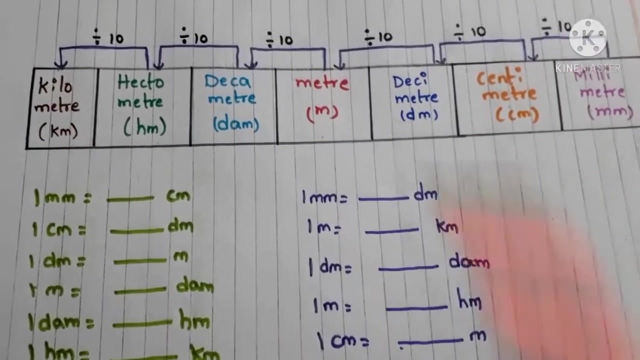 only one step Means that we have to multiply with 10.. So 1 decimeter is equal to 10 centimeters. Now let us see how to convert smallest units to highest units Here. to convert millimeter to centimeter, we have to divide with 10. Means that 1 millimeter is equal to 1 by 10 centimeters. 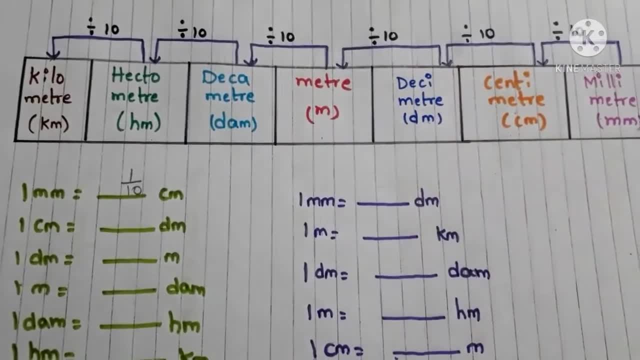 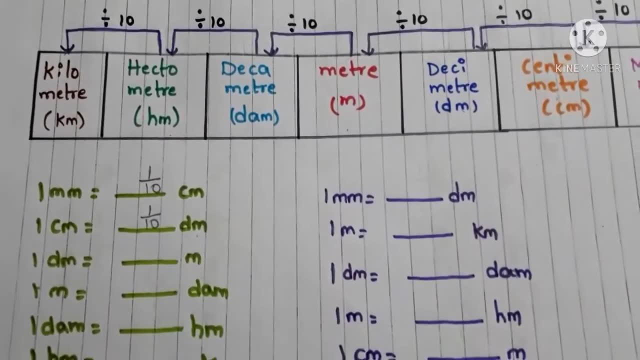 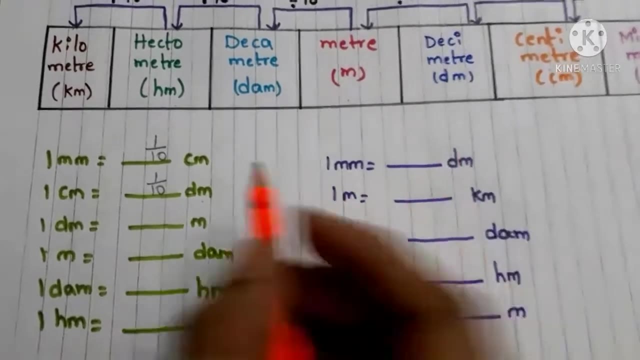 To convert centimeters to decimeters, we have to divide with 10.. Means that 1 centimeter is equal to 1 by 10 decimeters. To convert decimeters to meters, we have to divide with 10.. Means that 1 decimeter is equal to 1 by 10 meters. To convert meters into: 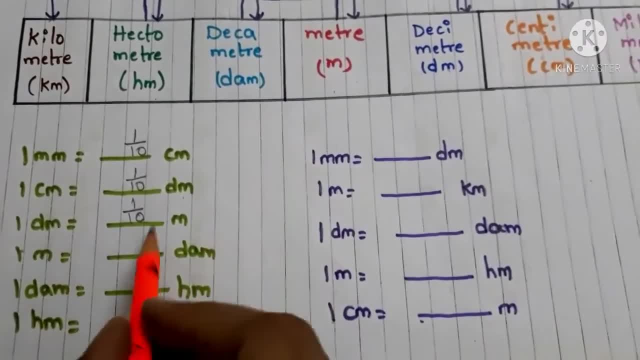 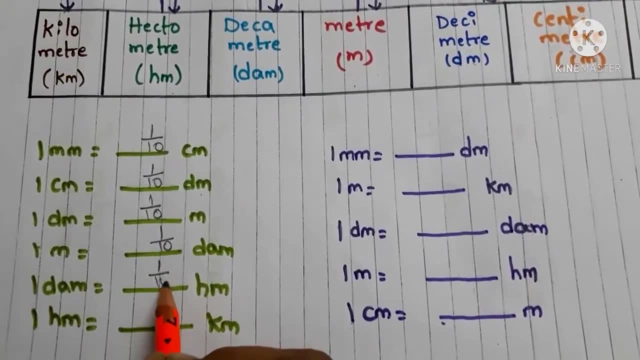 decameters we have to divide with 10. Means that 1 meter is equal to 1 by 10 decameters. Like that, 1 decameter is equal to 1 by 10 hectometers And 1 hectometer is equal to 1 by 10 kilometers. 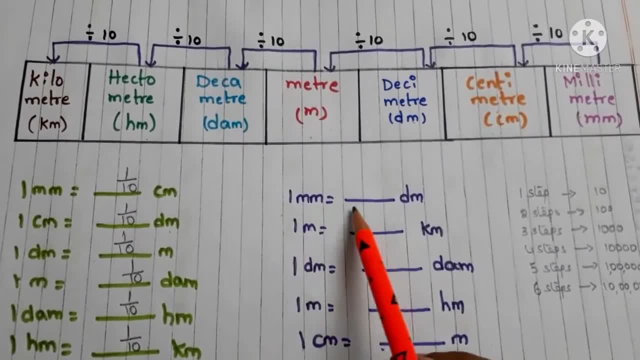 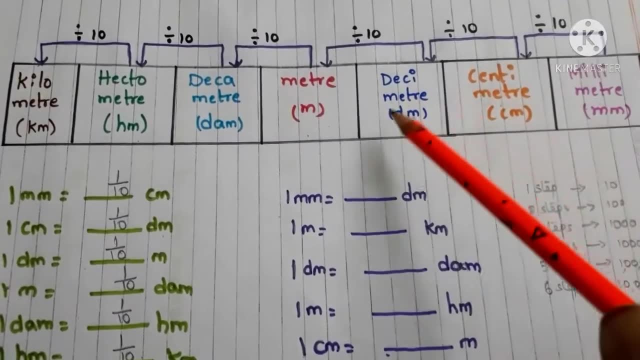 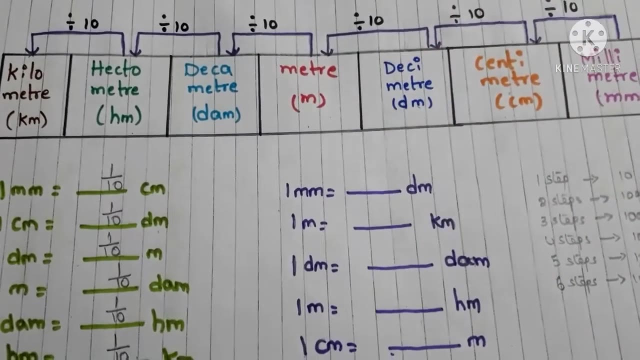 Now let us see: 1 millimeter is equal to how many decimeters. where is millimeter in the table? see, here it is. where is decimeter? here it is how many steps we have to move. one, two, two steps, right, so we have to divide with hundred means that one. 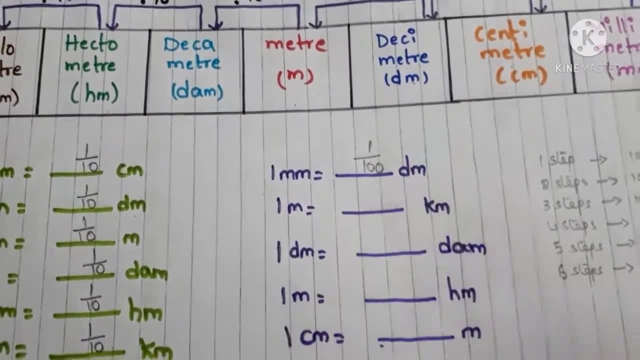 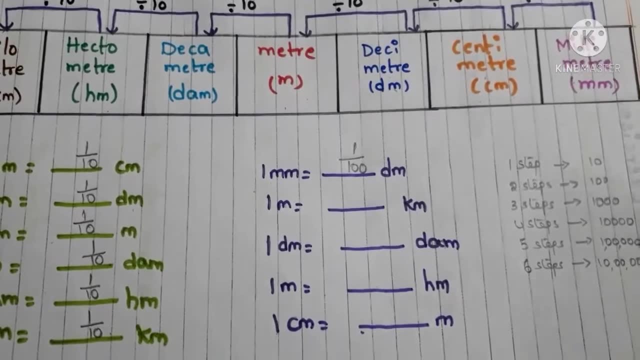 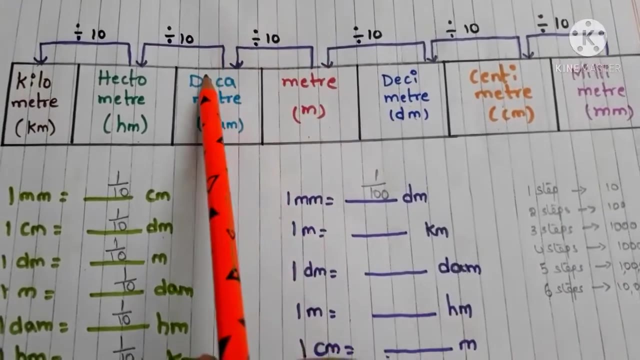 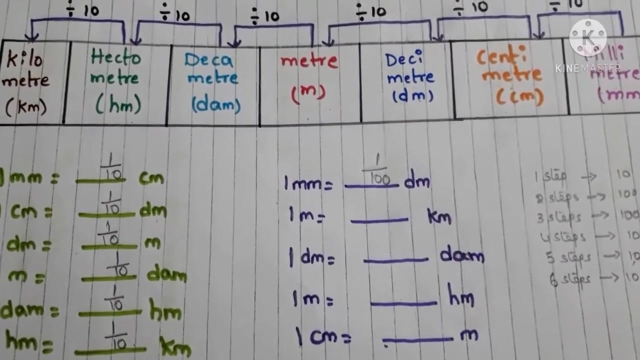 millimeter is equal to one by hundred decimeters. okay, let us see: one meter is equal to how many kilometers. where is meter? here it is. where is kilometer? here it is how many steps we have to move. see: one, two, three, three steps we have to move means that we have to divide with thousand. 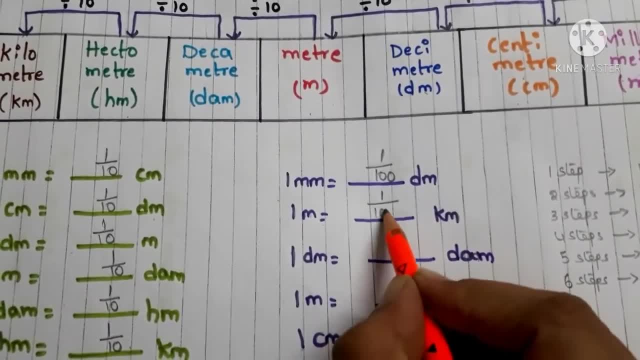 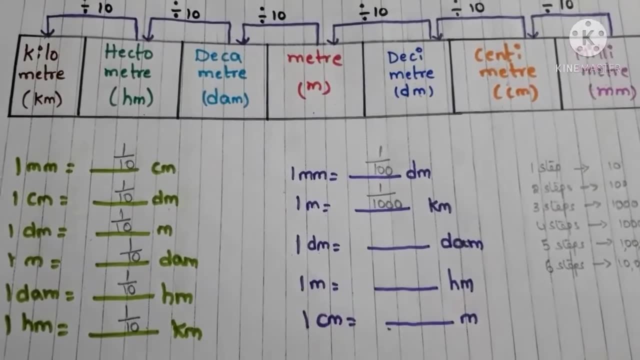 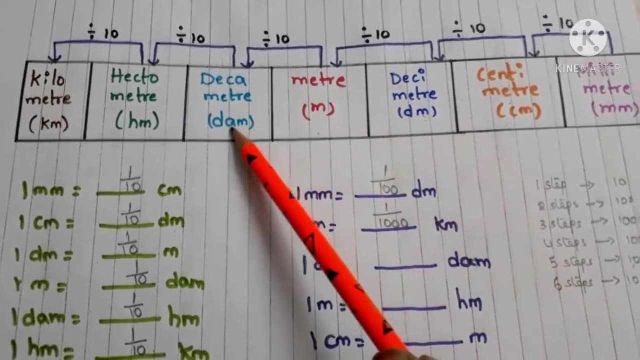 one meter is equal to one by thousand kilometers. okay, now let us see: one decimeter is equal to how many decimeters. where is decimeter meter in the table? here it is. where is decimeter? here? it is how many steps we have to move. see one. 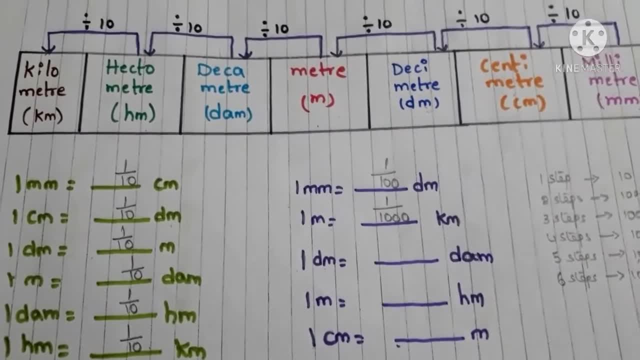 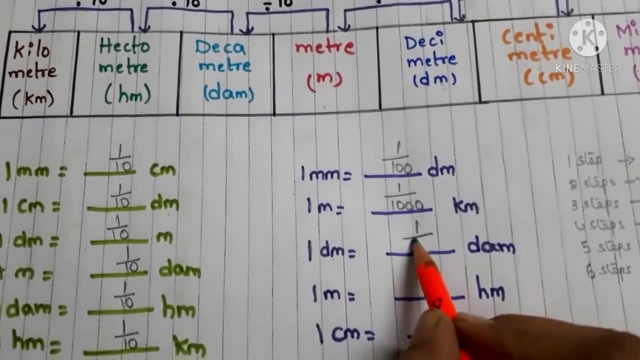 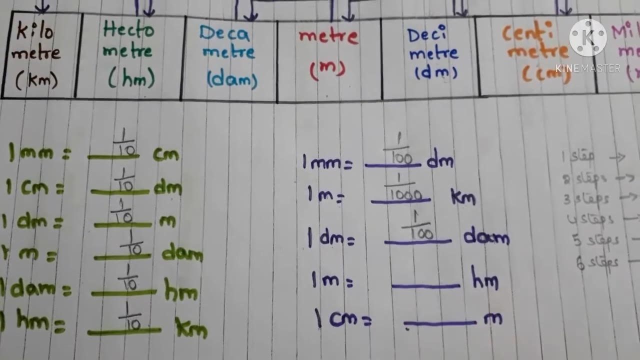 two, two steps we have to move means that we have to divide with hundred. so one decimeter is equal to one by hundred decimeters. okay, now let us see: one meter is equal to how many hectometers. where is meter? here it is. here is decimeter, here is decimeter. 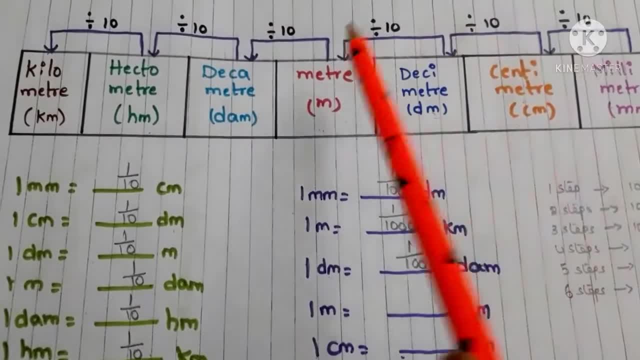 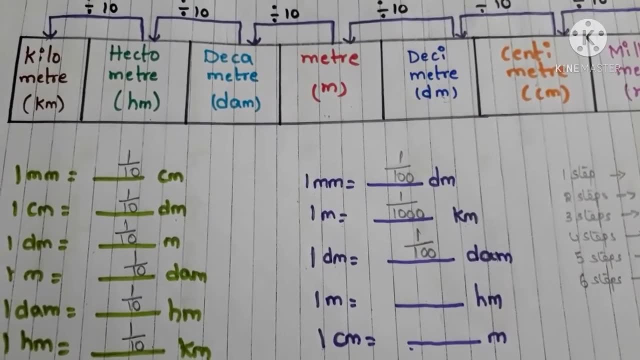 Where is hectometer Here? it is How many steps we have to move, See 1, 2.. 2 steps we have to move Means that we have to divide with 100.. So 1 meter is equal to 1 by 100 hectometers. 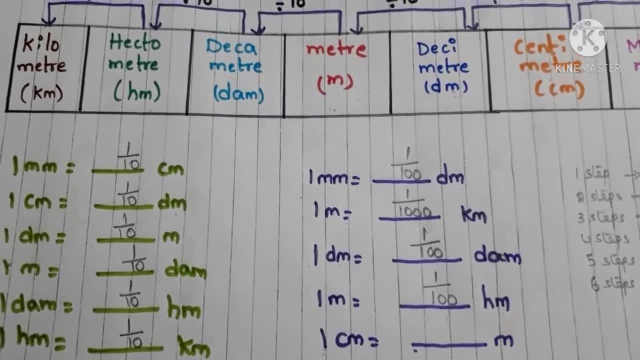 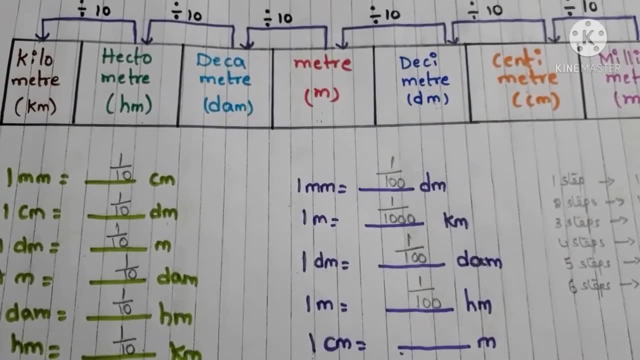 Okay, now let us see: 1 centimeter is equal to how many meters? Where is centimeter Here? Where is meter Here? How many steps we have to move? See 1, 2.. 2 steps we have to move. 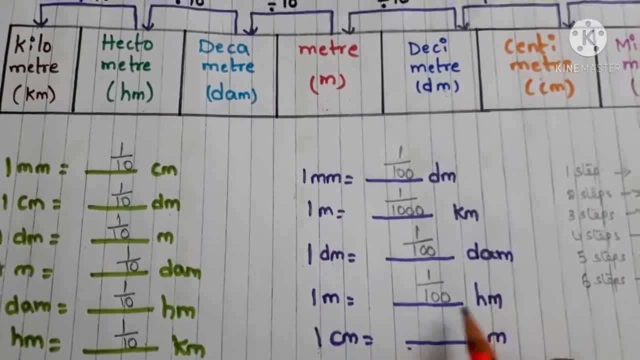 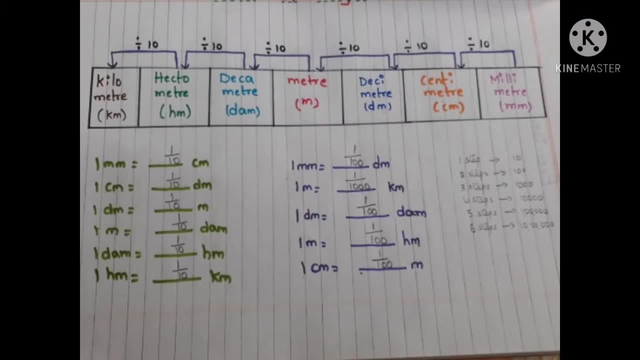 So we have to divide with 100. Means that 1 centimeter is equal to 1 by 100 meters. Okay, We will do the exercises in the next class. If you like my video, please like, share and subscribe.